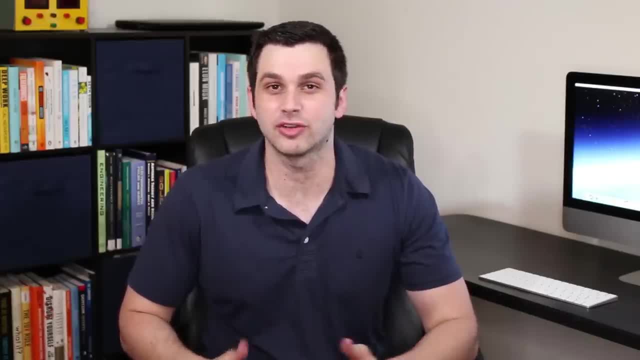 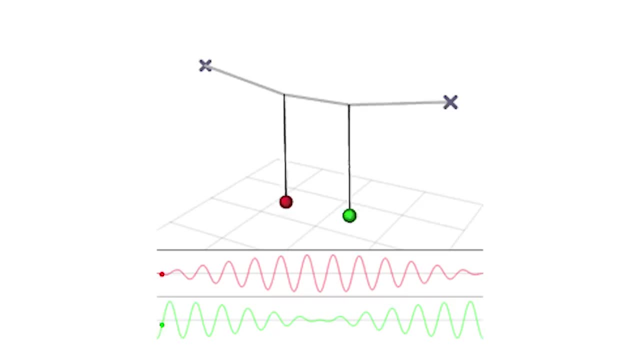 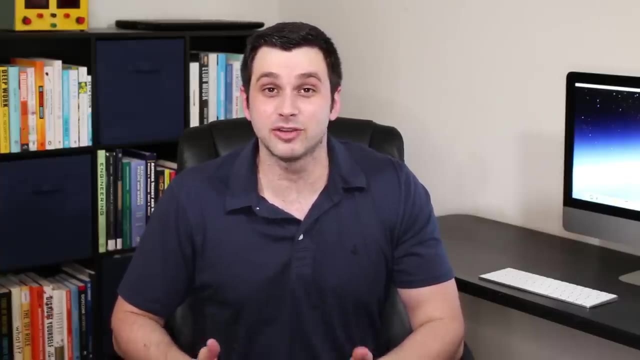 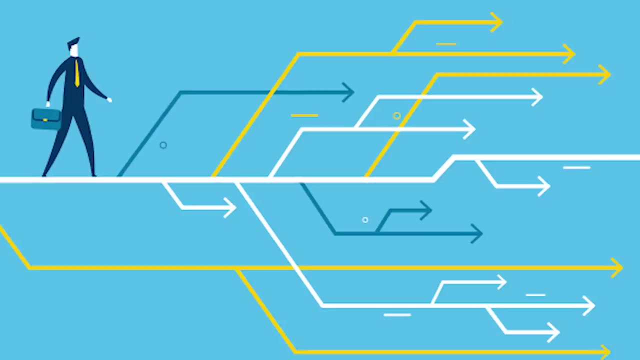 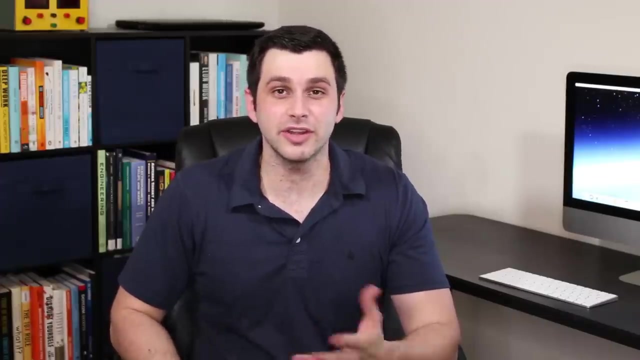 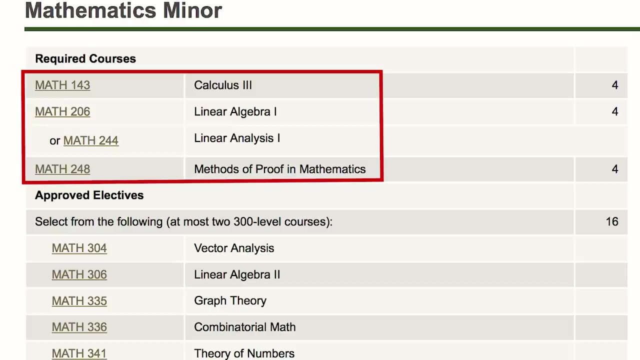 Math is one of the most popular minors to get, especially for people going into engineering or some kind of science. A lot of the math classes that most people don't get to take have applications in cryptography, complex dynamic systems, higher dimensional surfaces, and so on. Whether you want to pursue some math degree later on or you just want to expand your knowledge, getting a math minor is one way to help with that. Remember, a minor is just where you take a few extra classes in a certain field. It's not going to open up a huge range of job opportunities and it's not required, but it can help your resume at times and provide a good foundation in other topics. So let's look at the requirements at my school if you want to get a math minor and then I'll talk more about the classes. These are the three required courses you have to take. There's Calc 3, which means of course Calc 1 and 2 are also required, and then there's Linear Algebra. Those two classes are taken by all engineers, computer scientists, and physics majors regardless. So look at that, you're already on your way to a math minor if you study one of those other majors. 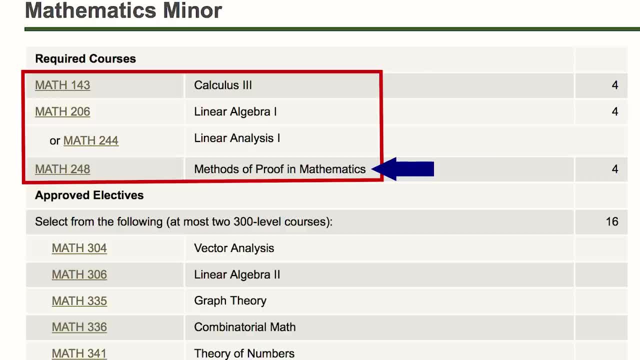 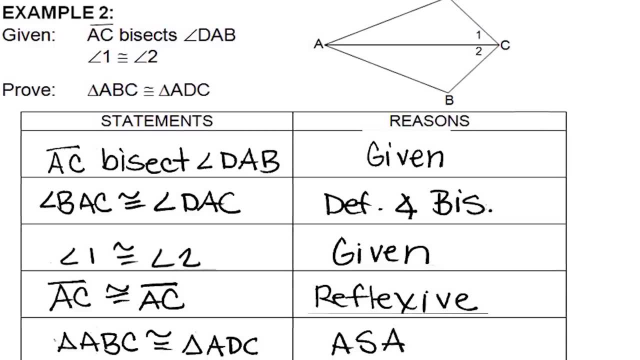 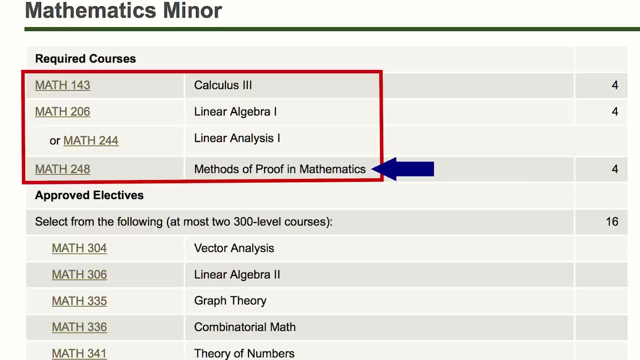 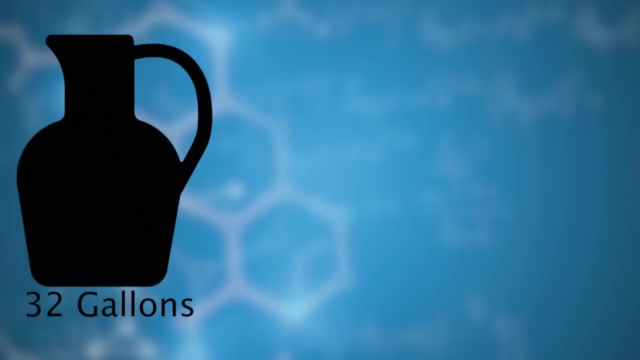 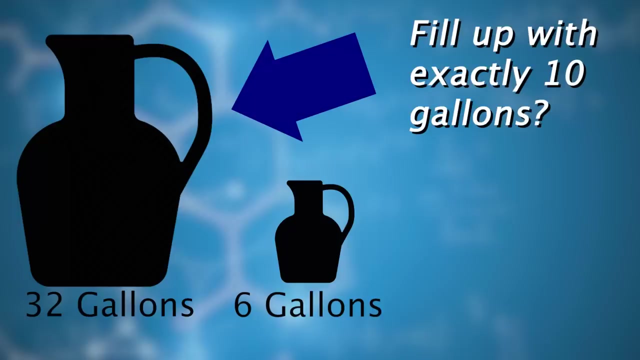 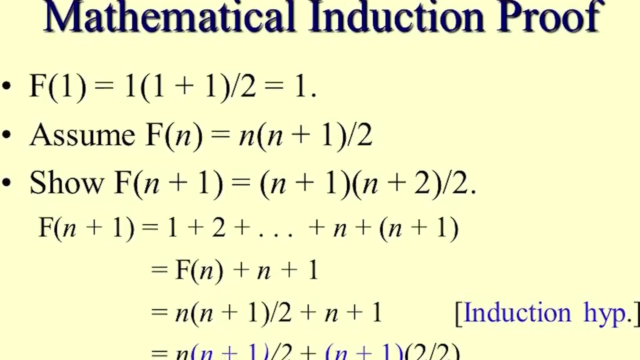 The next requirement is that you're not required to take a math major. The required class is your proofs class. As I've said before, this class did not sound fun to me years ago because the only times I had done proofs were in geometry, and honestly side angles, side triangles, and two table proofs bored me. If that's you, don't worry. This class is much different and I finally learned I actually do find those proofs interesting. This class is where you learn how to prove that the square root of 2 is irrational. Or you learn tools for proving whether using only a 32 gallon jug and a 6 gallon jug you can fill up the 32 gallon one with exactly 10 gallons, assuming you had infinite water, which involves number theory or the study of integers, a foundation for cryptography. And there are plenty of specific proof techniques you'll learn in order to do these problems. This class is required because lots of upper division classes have it as a prereq. 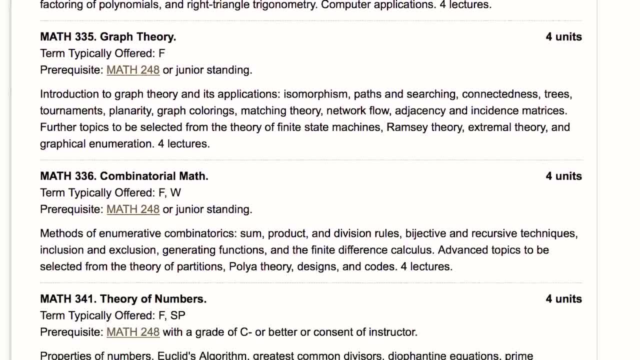 Additionally, lots of high level math courses, especially in pure math, involve rigorous proofs. 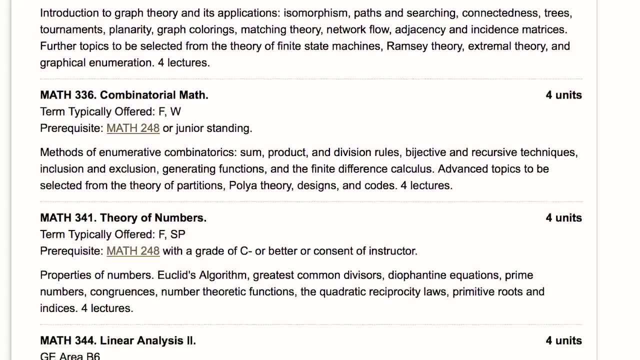 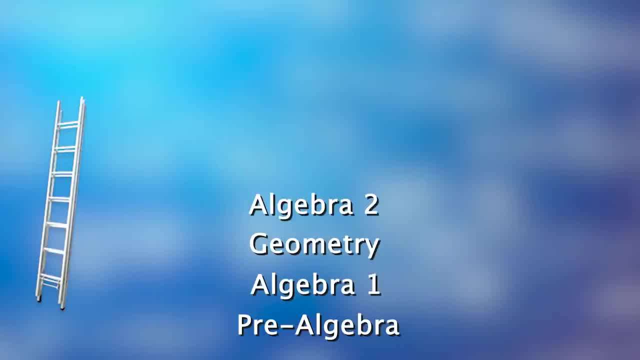 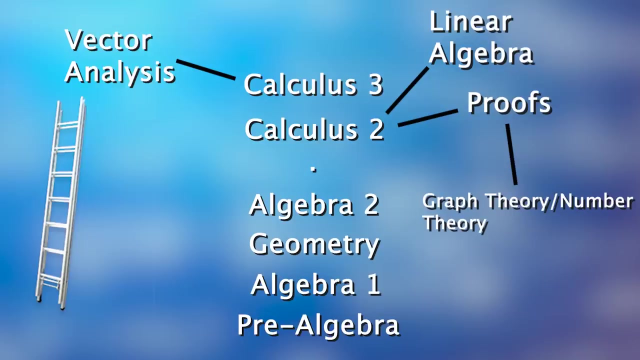 Now before I move on to the other classes, I want to emphasize something. Throughout most of school, math is like a ladder. You get to pre-algebra, then jump to Algebra 1, Geometry, Algebra 2, Pre-Calc, and so on. You always need one before the next. Once you get to college though, it becomes more like a tree. For example, after Calculus 2, at least at my school, you can take Linear Algebra and you can also take a proofs class that most majors don't take. After proofs, you can take Graph Theory and Number Theory. After Calc 3, you can take Vector Analysis and then after that Differential Geometry. Or after Calc 3, you can take Numerical Analysis. I could go on, but hopefully you get the point. And note, these are specific for my school. Others 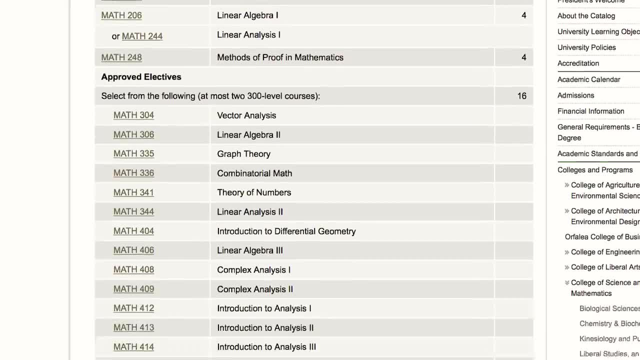 are different in terms of their prereqs. But okay, now let's get into all these other classes. 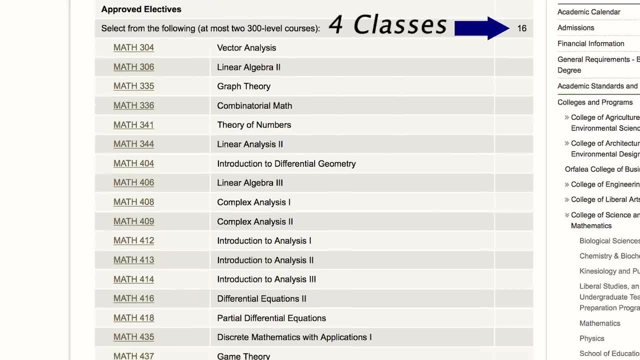 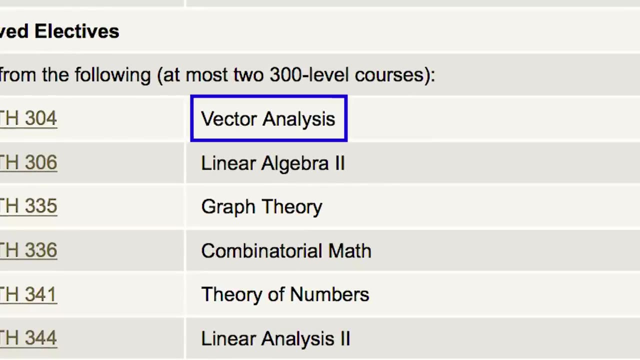 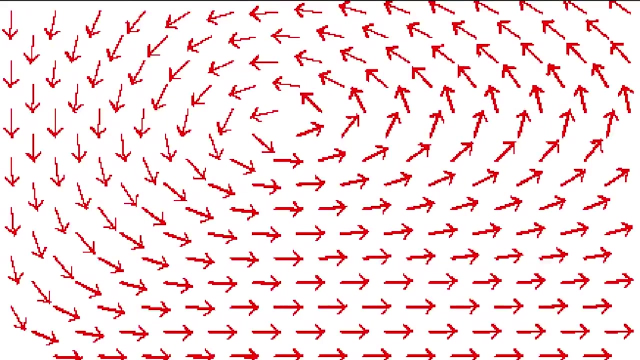 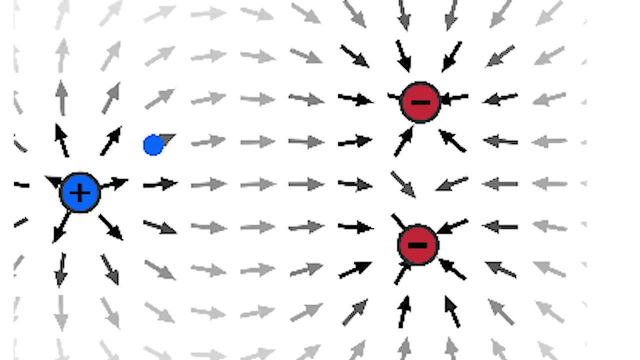 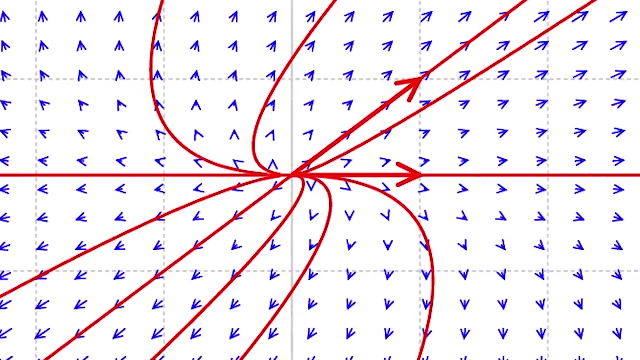 As you can see, you're required to take 16 units, which means 4 of these classes. And you can pick whichever ones you want so long as you have the prereqs. I'll go over a few and explain who they might be right for depending on your major and interests. The first one I'll discuss is Vector Analysis. This class goes into depth on Green's Theorem, Stokes' Theorem, and the Divergence Theorem. For those who have not taken Calc 3 yet, if for example you have a complicated vector field, a whirlpool of some fluid, and you move an object through it in some weird path, it can be difficult to calculate how much work is done on it or its final velocity. The techniques you use in this class simplify that process. Whether it be a magnetic field, electric field, gravitational field, and so on, when something moves through a field of complex forces, we need vector analysis to analyze what will happen. 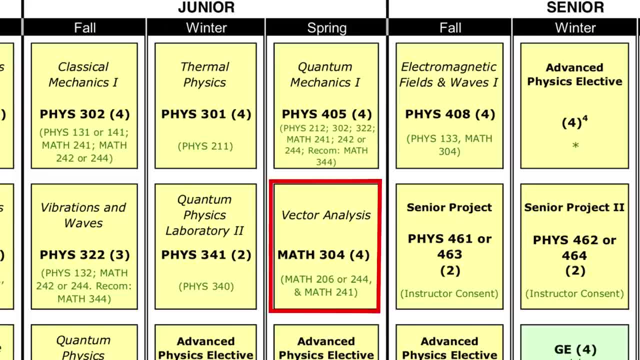 This class is required for physics majors at my school, and is a good one to take for electrical engineers who are going into wireless communications because electromagnetic waves are very sensitive to the field, and you will do vector analysis. 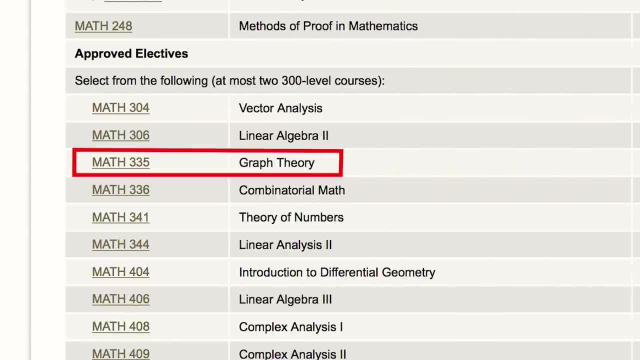 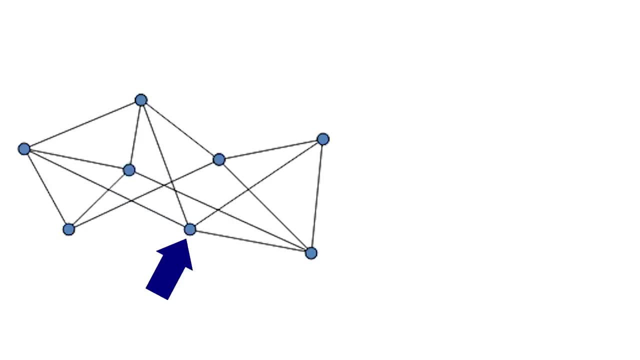 Next one is Graph Theory. This class is great for computer scientists who want to learn more about the field, because they already do learn some in other classes. Graph theory is not the graphs you're thinking of. It's when you have a bunch of nodes, or dots, and lines that connect them, or edges. This could represent a network of computers that are connected where you want information to take the shortest path from one point to another. Nodes could represent classes, and edges could mean at least one student is in both classes. Like this edge means at least one person is in both this chemistry class and english class. If you want to develop 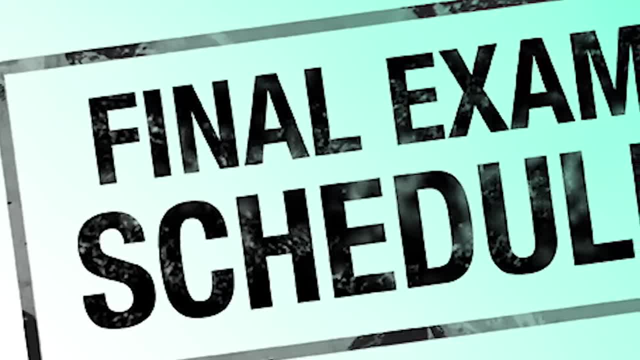 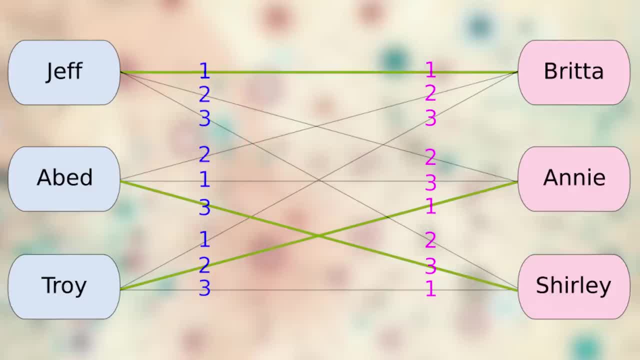 a scheduling algorithm for finals week such that no one has conflicting times, you would need graph theory. Whether it's determining shortest paths, compatibility according to a dating profile, or an algorithm to rank chess players based on who's played who, you need graph theory to help with these. 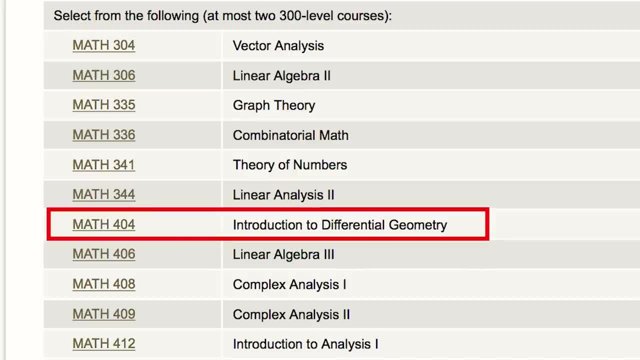 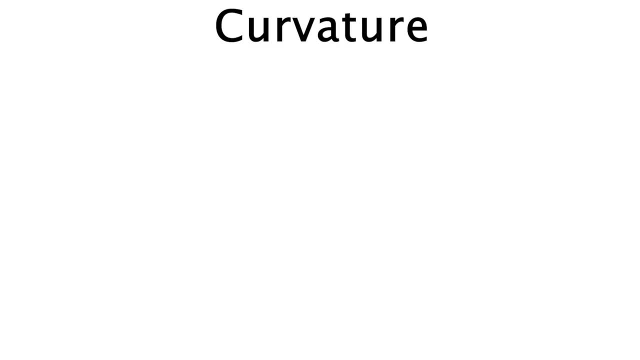 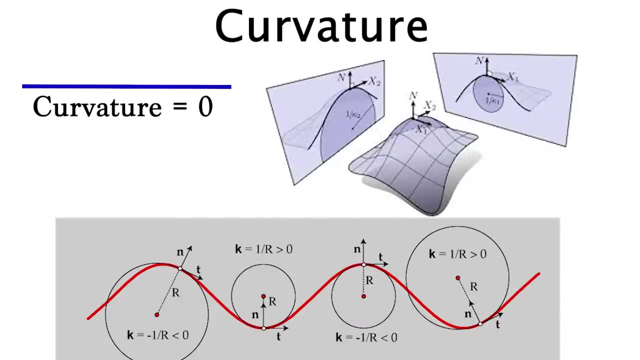 Next up is Differential Geometry. This uses calculus techniques, among a few other prereqs, to analyze problems in geometry. You'll analyze the actual curvature of certain shapes and surfaces. If a line can be said to have zero curvature, since it's straight, how can we quantify the curvature of other shapes and surfaces? Well, it involves calculus. 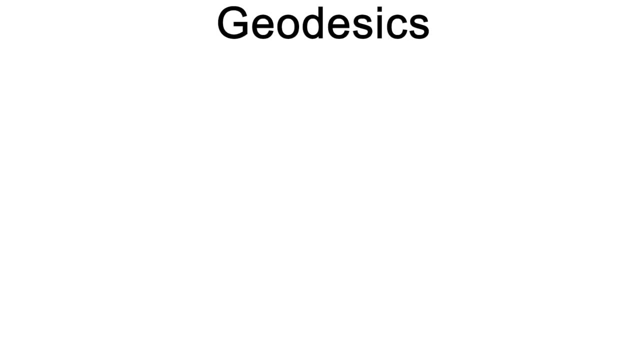 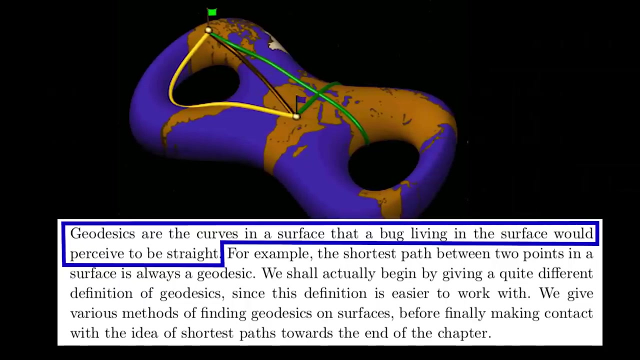 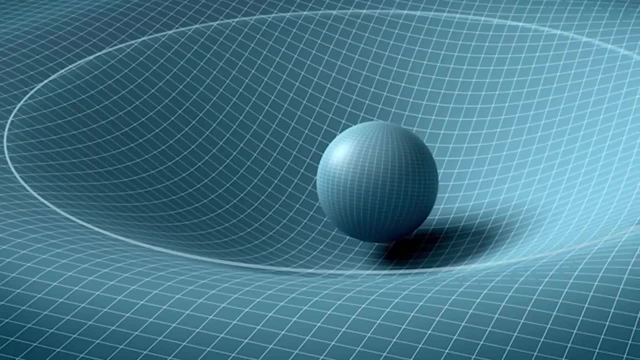 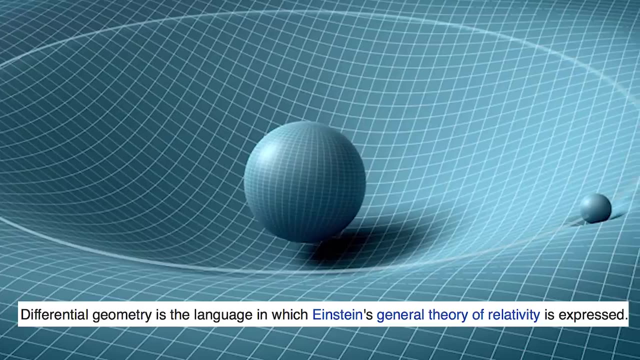 This class is fairly advanced, but it dives into depth on complex curves and surfaces. The concepts are a foundation for understanding Einstein's general theory of relativity and the curvature of spacetime. In fact, they say differential geometry is the language of Einstein's general theory of relativity, but it has plenty of other applications as well. 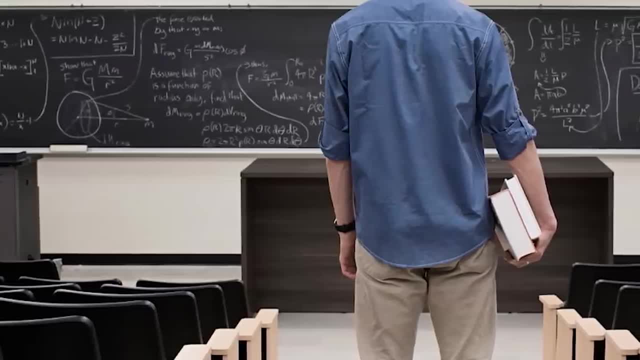 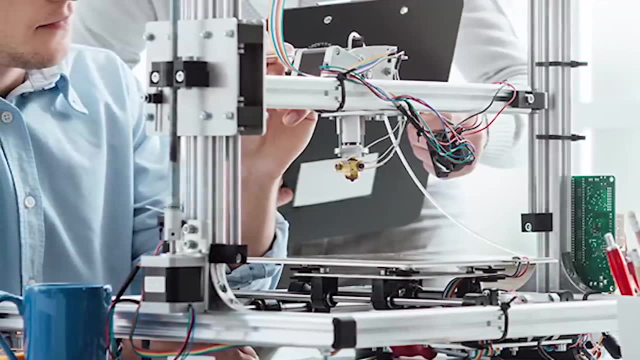 Differential geometry is really important for physicists going on to grad school, but in a bachelor's you may or may not see it. Then the class can be interesting for engineers, but is not something you will likely need during your career. 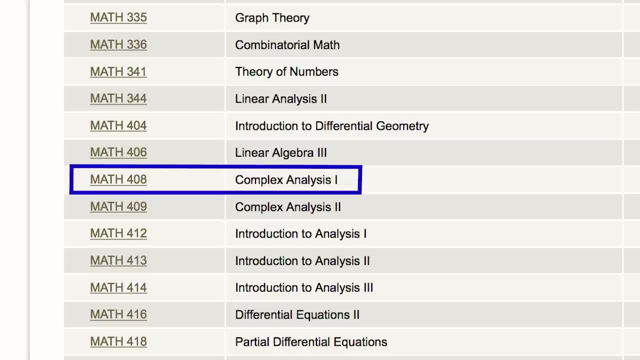 Moving on, complex analysis is a class dedicated to complex numbers, or numbers with an imaginary component to them. These actually do have a ton of applications, especially when analyzing waves of some sort, complex numbers will come up. 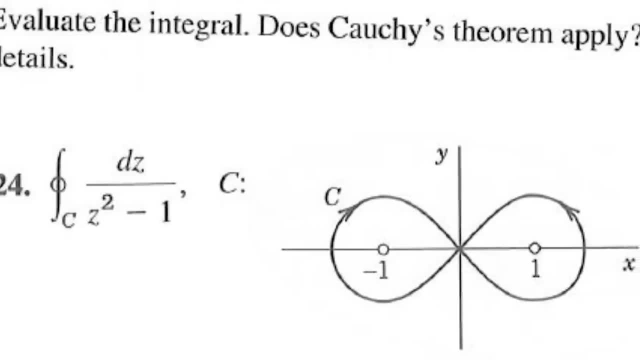 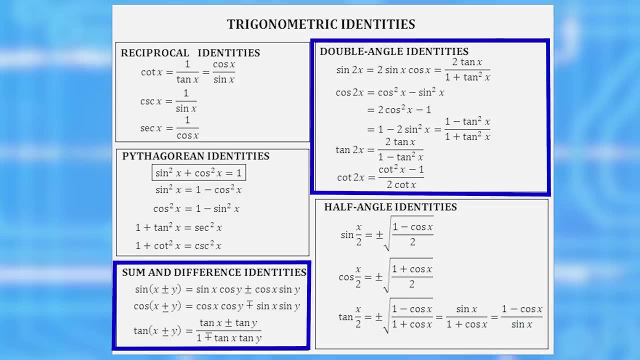 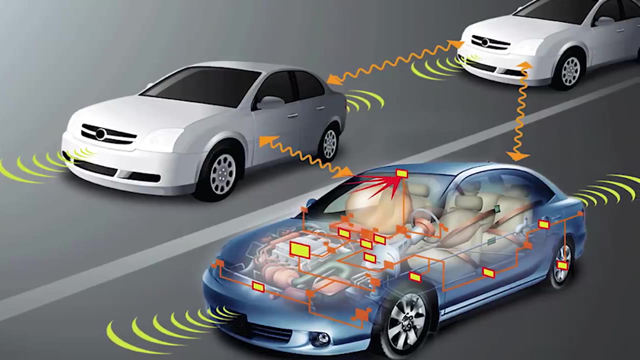 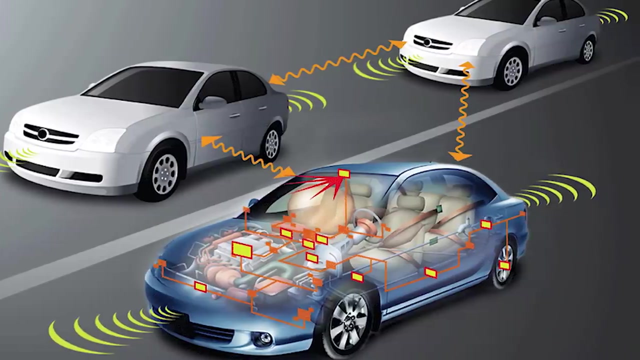 You'll learn how to do calculus in the complex plane, and when I took this class actually on day 1 and 2 we proved a bunch of trig identities you learn in Algebra 2 or PreCalc using complex numbers and Euler's formula. Complex numbers apply to signals, quantum mechanics, relativity, control systems, and several other fields. Physics majors and electrical engineers would benefit from this class the most, and at many schools it is required for one or both of those majors. 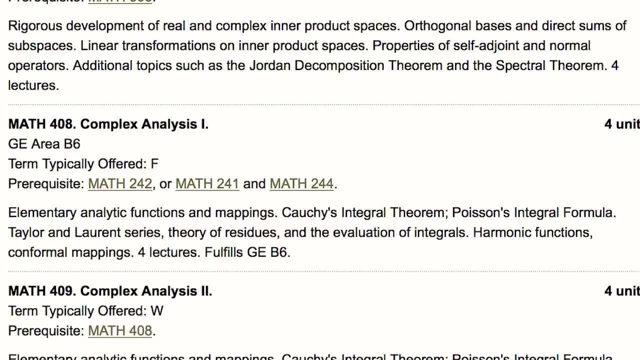 The class does go into much more depth than most would need at a bachelor's level, but it will expand your knowledge on a subject that most people really never learn. 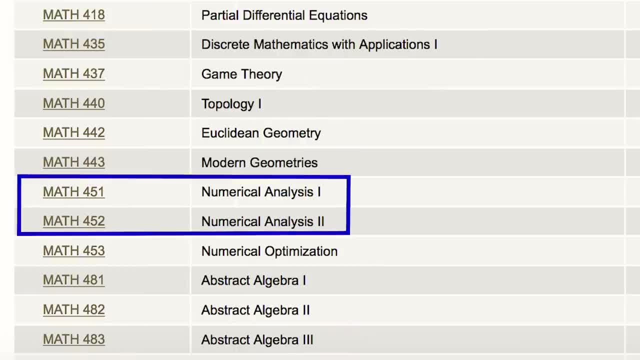 Next is numerical analysis. This is great for engineers and physics majors and is very applied. Many majors require it, but as you can see you have the option to take more. 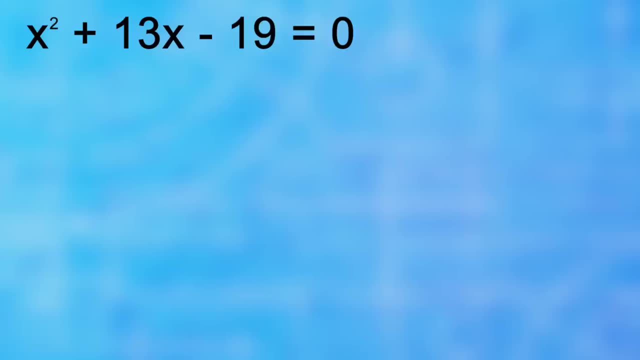 I've described this in other videos, but I'll say it again. If you were asked to solve this, you could just plug in the numbers to the quadratic formula and have 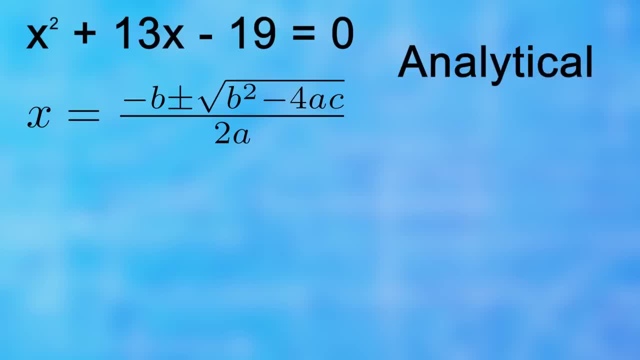 the exact answer come out every time. This is called an analytical solution, since it's exact and involves a formula. If you were asked to solve this though, 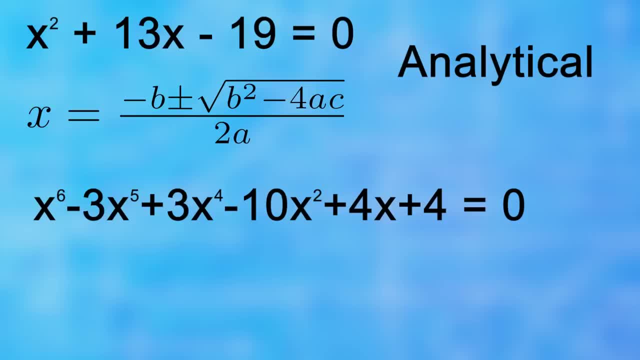 and you were not given a calculator or anything, the best you could probably do is guess and check. 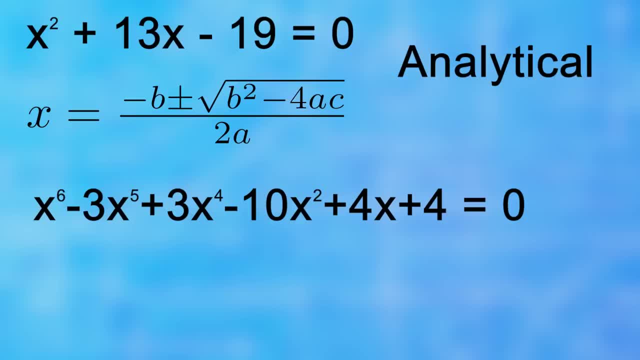 But we still need ways to solve these problems fast and efficiently, especially when they represent real world situations. So we use numerical methods or numerical analysis to solve them. There are algorithms and methods to approximate solutions like this to very high accuracy, and with enough computing power, like an actual computer, 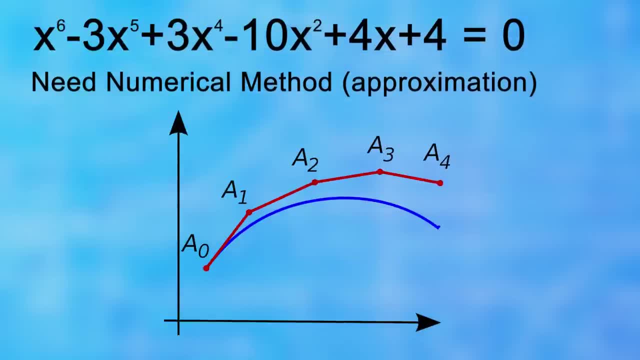 you can get basically an exact answer. For example, Euler's method can approximate the curve that is the solution to a differential equation, which many people learn in Calc 1 or 2. 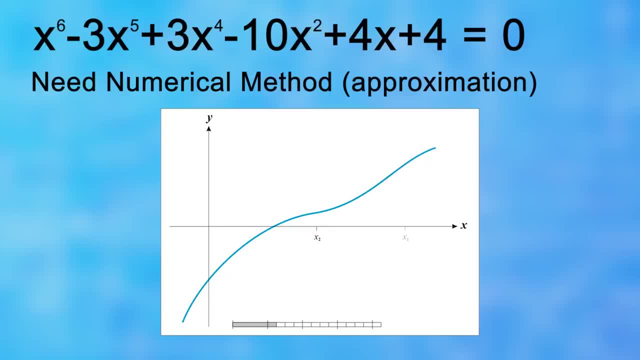 Newton's method can find the zero or x-intercept of a curve after running its algorithm a few times to narrow in on the answer. And this can be used to solve the problem from before. 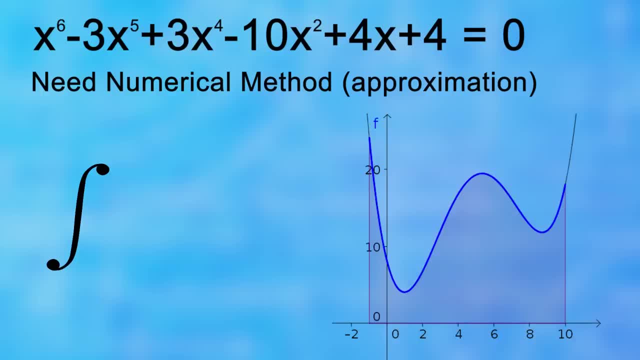 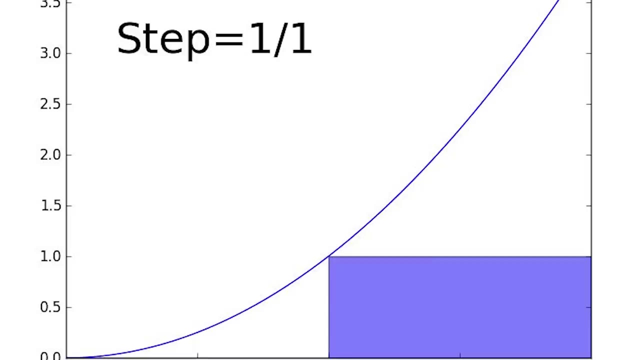 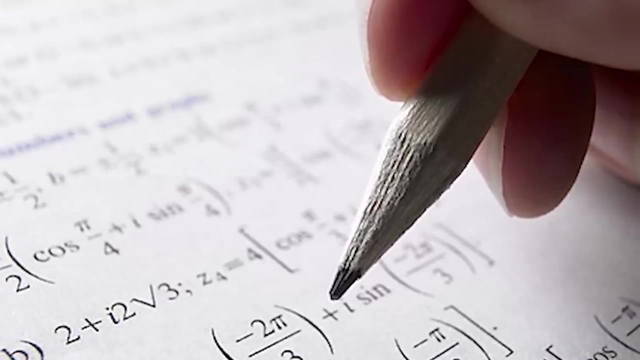 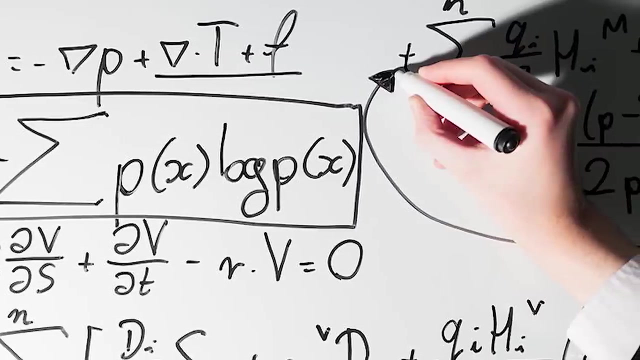 Then for those who have taken calculus, you know the integral tells you the area under the curve. But when it is literally impossible to integrate something, we can estimate the area under the curve using rectangles, trapezoids, or even a number of other factors. So if you're a computer, you know that you need to know the area under the curve. And if you know the area under the curve, you know that you need to know the area under the curve. And if you know the area under the curve, you know that you need to know the area under the curve. These are other numerical methods. They're not exact, but a good approximation, and given enough time, you could get extremely accurate. We spend so much of school learning all this math that we can do by hand, but when it comes to real world systems, more often than not, you cannot just come up with an equation and solve it on a whiteboard to determine the stress on an object given some force. 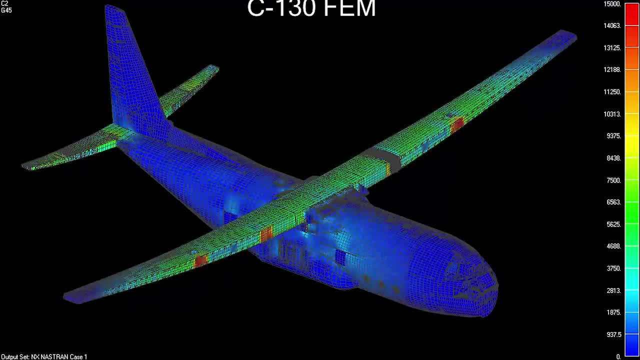 We need computers to do the work, and those computers need to be programmed with mathematical algorithms to come up with solutions. 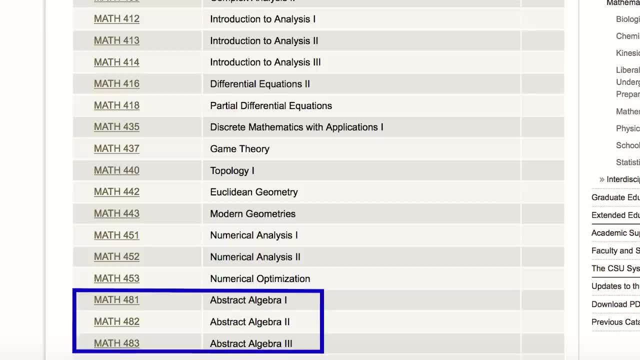 Next, you'll notice three classes on Abstract Algebra, and three on Intro to Analysis, often known as Real Analysis, a class on real numbers or numbers without an imaginary component that we all know of. These are really big classes for math majors, but are more on the pure mathematics side. Especially as an engineer, these are good if you want to challenge yourself and experience some courses in pure mathematics, but don't really expect to use the information you learn. Pure math courses are more about solving problems within math, rather than learning math to solve problems in physics or mathematics to solve problems in physics or mathematics. 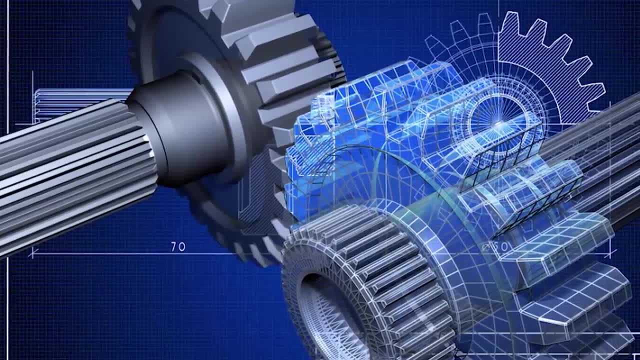 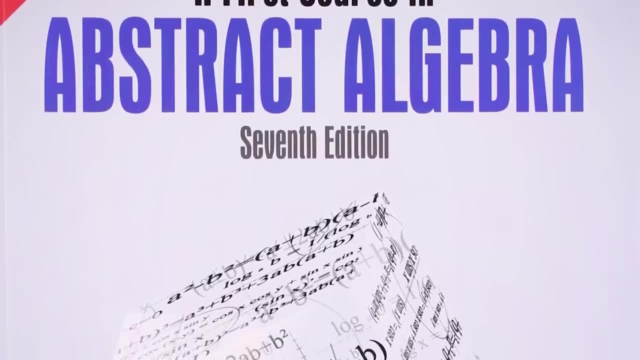 So again, don't expect many applications. Abstract Algebra, for example, does have applications that physicists can encounter, especially in grad school, but that does not happen until you reach a certain level, which won't really apply to a majority of people watching, most likely. 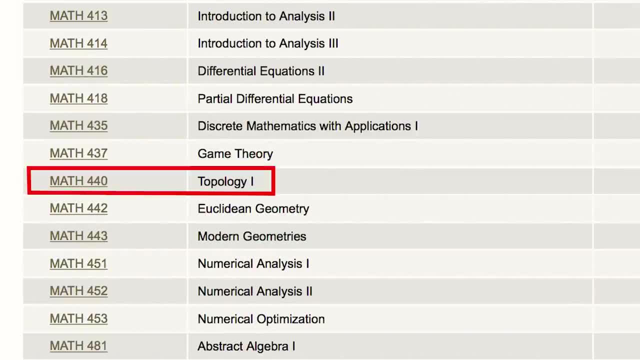 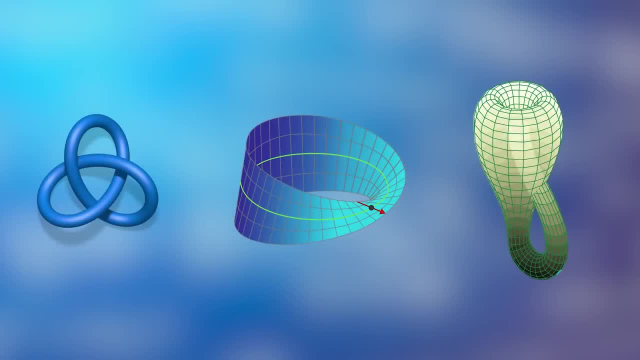 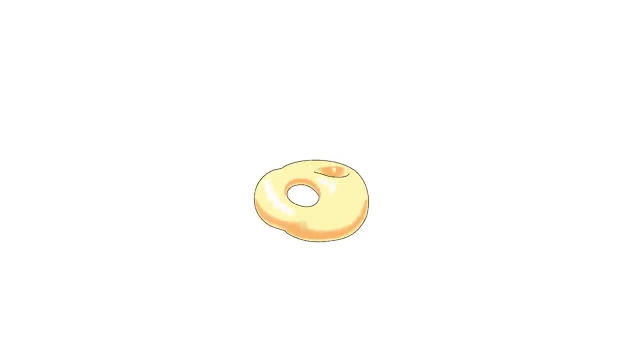 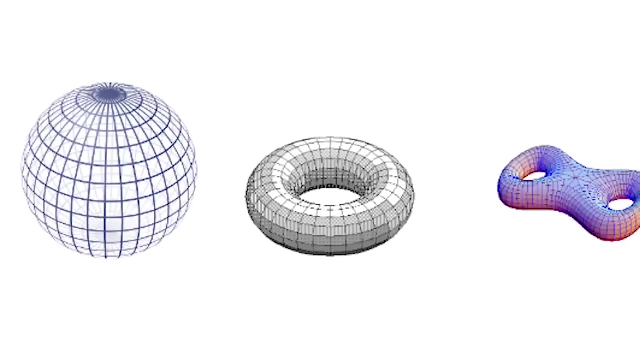 And lastly, another huge field of math is topology. This is kind of like the study of shapes, but you analyze much more abstract shapes that are preserved under certain deformations. So in topology, if you can morph one object into another without tearing it, filling in holes, or anything like that, those objects are considered topologically the same. In this class, you learn about connectedness and continuity. Properties like how many holes an object has matters, whereas angles or lengths don't. That's more for geometry. 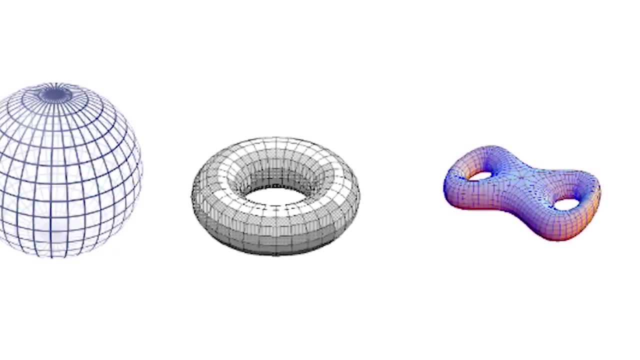 And in this class, we'll even get into higher dimensional objects. One of the most famous shapes you learn about is the Mobius strip, and there's actually a fun demonstration for it that 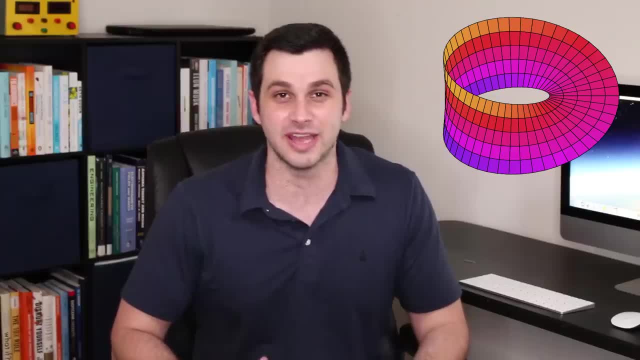 I want to show you guys. A lot of topology teachers may do this on the first day, but it is a very simple one, so if you've seen it, just skip to this part of the video. 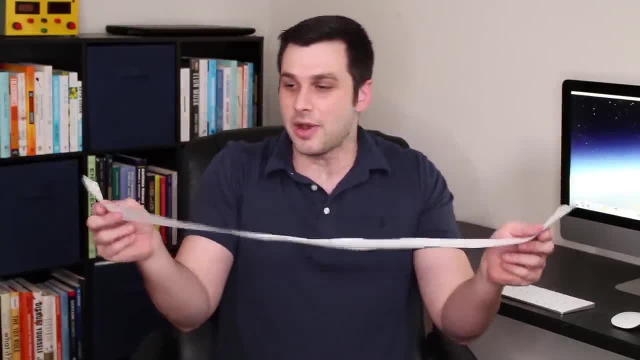 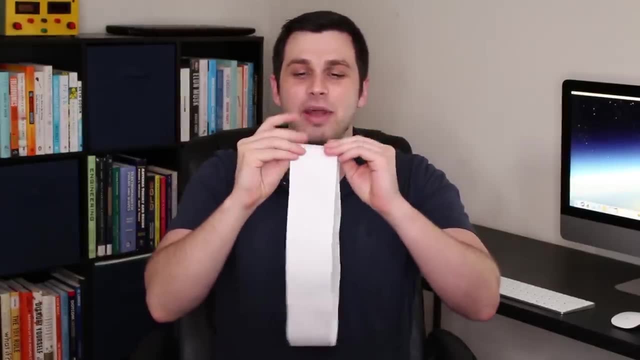 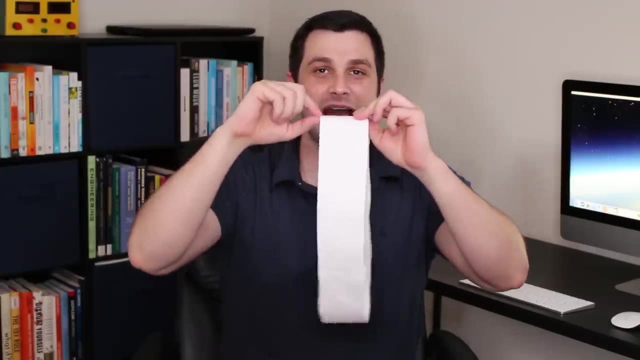 Okay, so here we have a long sheet of paper. Now, if I were to connect these two ends, this shape is nothing special. It's like the shell of a cylinder, the outside. And if I were to cut down the middle all the way around until I got back to the original cut, it should be no surprise that this thing would split in half and just fall apart into two pieces. 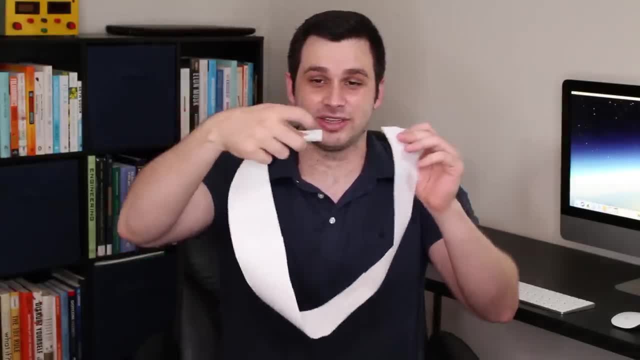 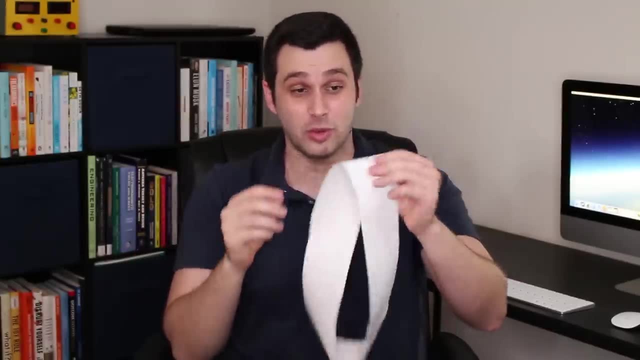 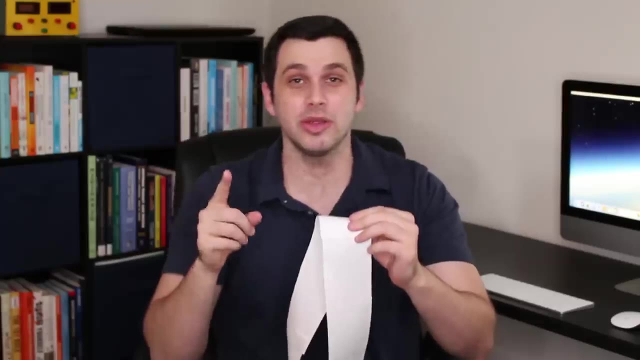 Now the question is, if I put a half-twist in this and then connected it, what's going to happen? So this is a Mobius strip for the most part, and the question in the demonstration is, if I cut down the middle all the way around to the original, what is going to happen? So comment below what you think is going to happen while I tape this up. 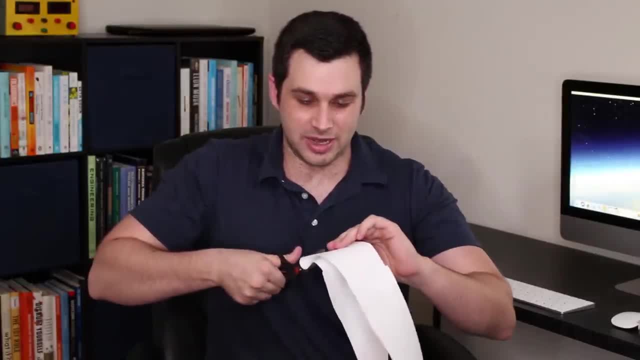 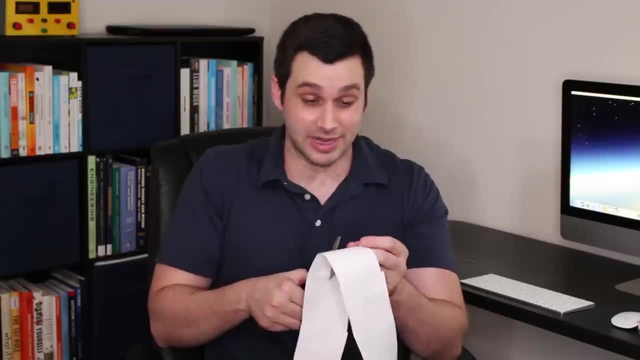 Okay, so what I'm going to do is just make a little cut right here in the middle, and again I'm going to go all the way around until I get back to this original cut. So again, comment below. We'll see what's going to happen. 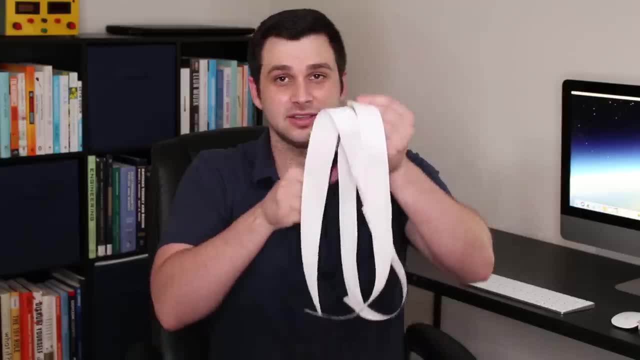 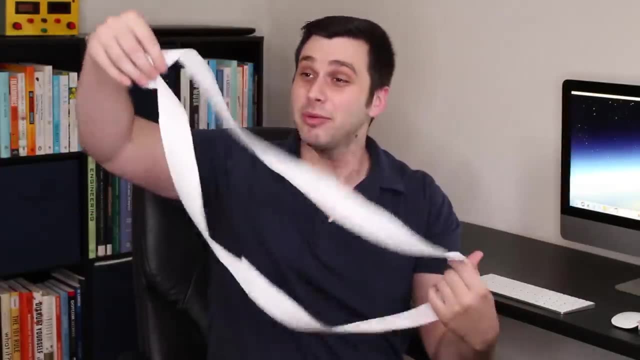 All right, here we go. Last cut, and it is still one piece. So if you were able to guess this, then congratulations because I definitely 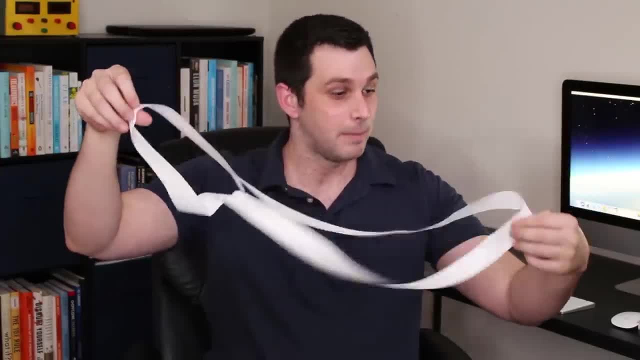 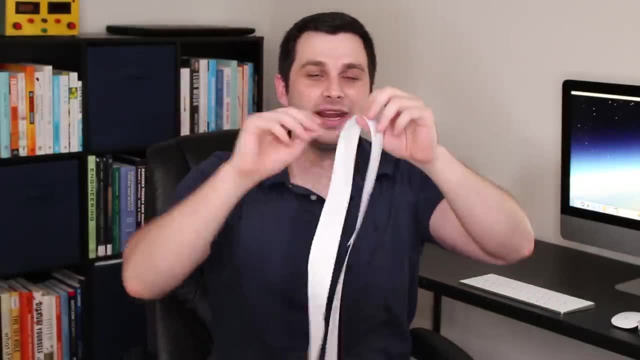 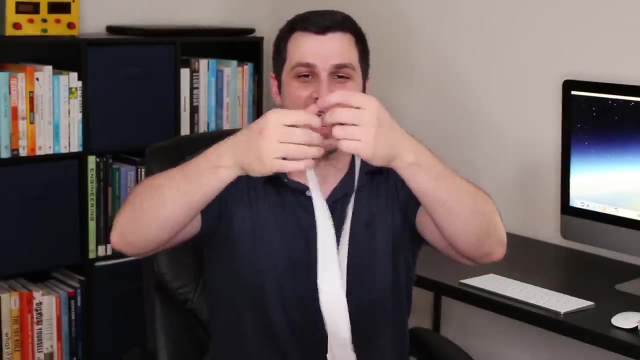 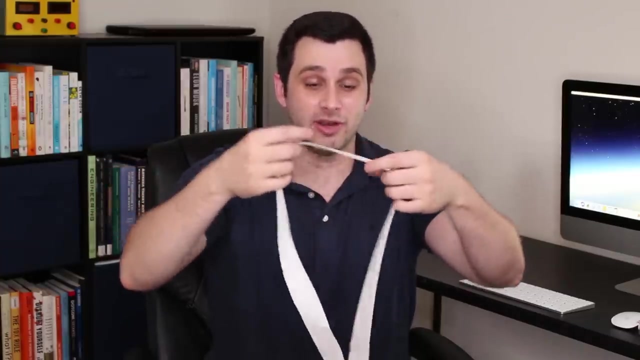 did not expect that to happen the first time I saw this. But if you did get that, try to go a little deeper. Is this still a mobius strip remember when i did the one half twist and connected them that's what a mobius strip was so if we were to cut this i'm not going to do it if we were to cut this and then i were to unravel it till it was just a flat piece of paper again would it involve one half twist to undo it or would it involve more and the answer to that is it would involve more 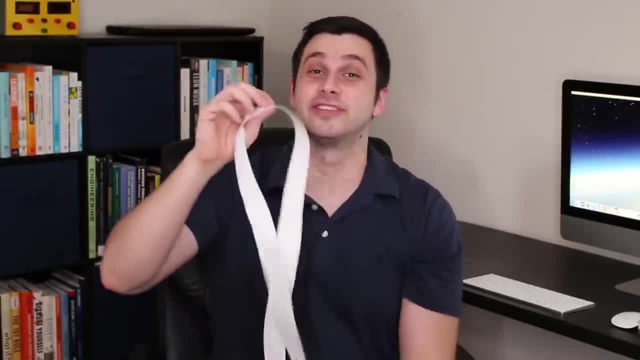 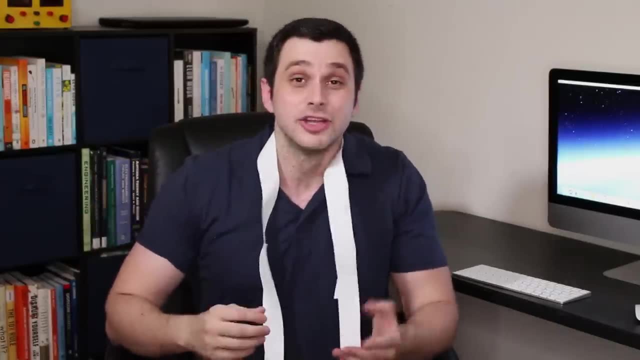 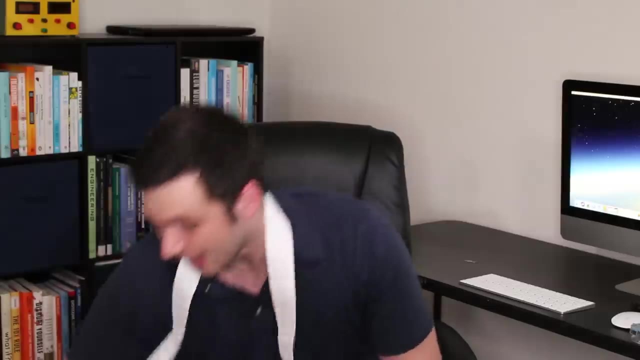 there's actually two full twists in here so no this is not a mobius strip and for the guys who cannot afford to buy a necklace for your girlfriend there you go it's multi-functional so you just learned something and i saved you a trip to the dollar store now for those who did not guess that last one correctly i will do one more presentation but this one's a lot weirder 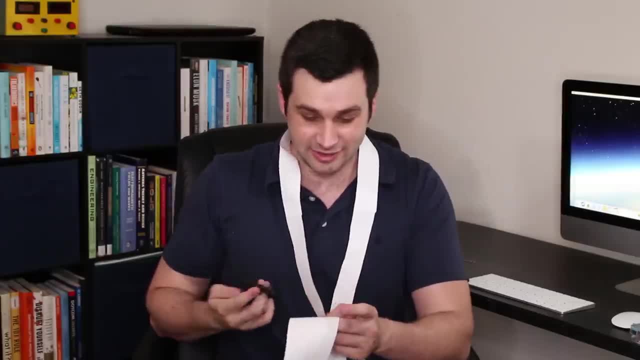 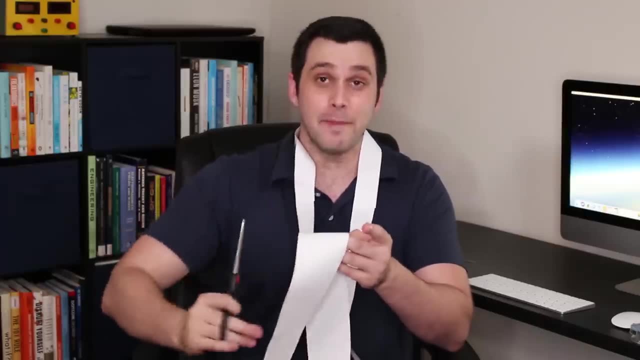 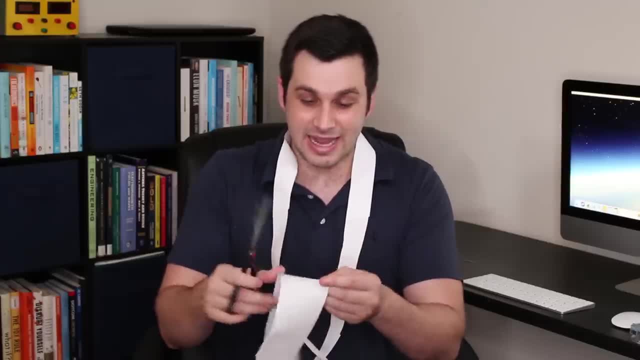 third of the way third of the way instead of halfway and again comment below what you think is going to happen here we go 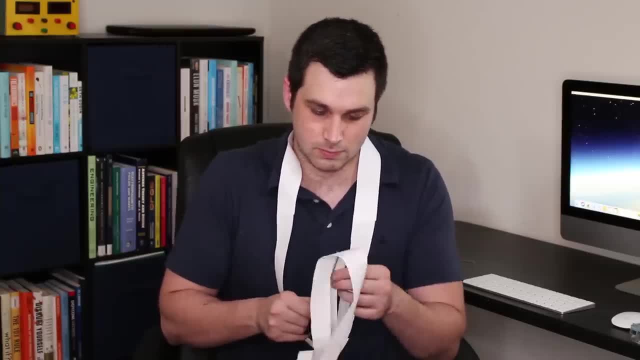 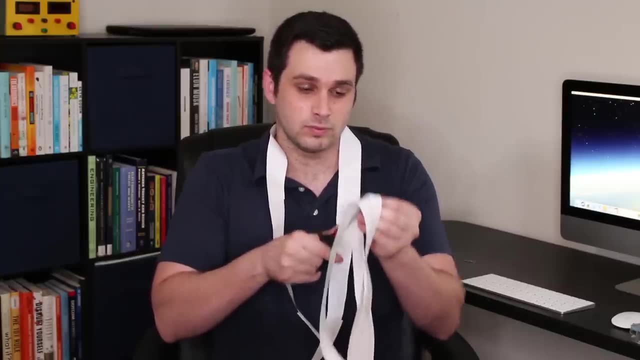 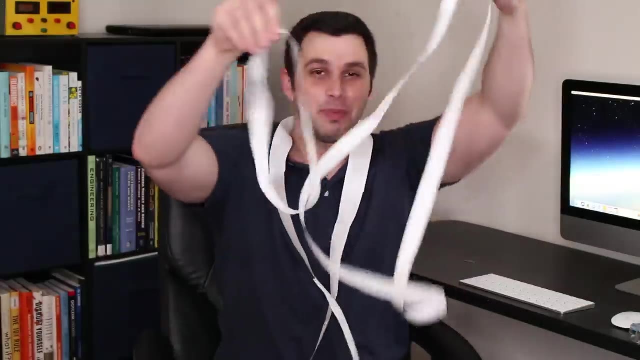 all right and again last cut here we are all bets in and here's what we have we have two pieces connected kind of like rings hopefully you can see this 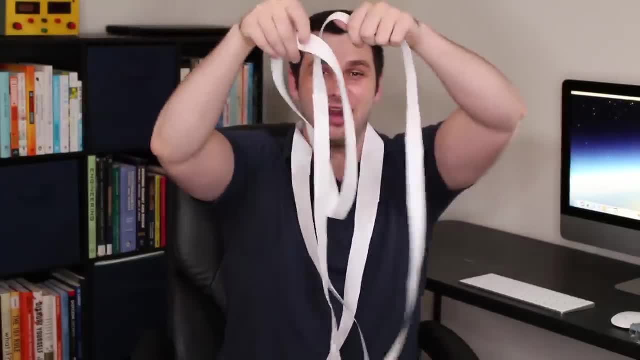 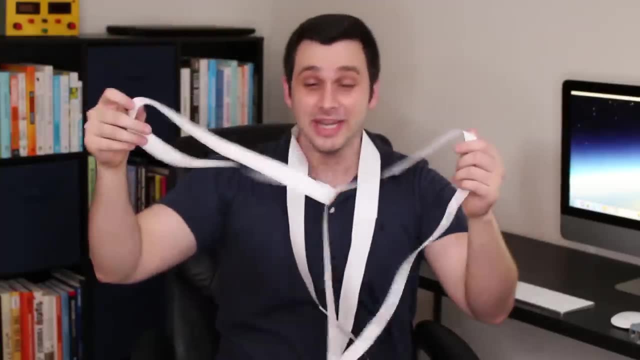 we've got a smaller piece and a much larger piece and they are yes their own pieces but they are uh connected so if you did guess that then again congratulations i had no clue that 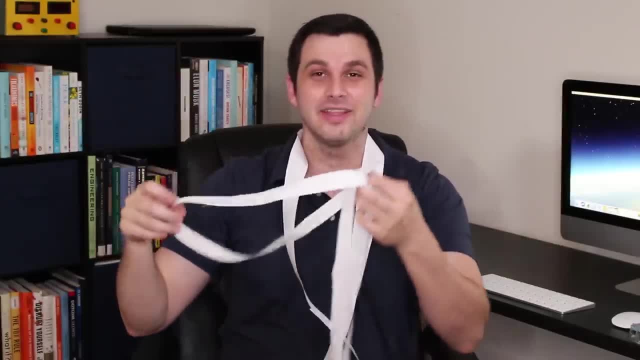 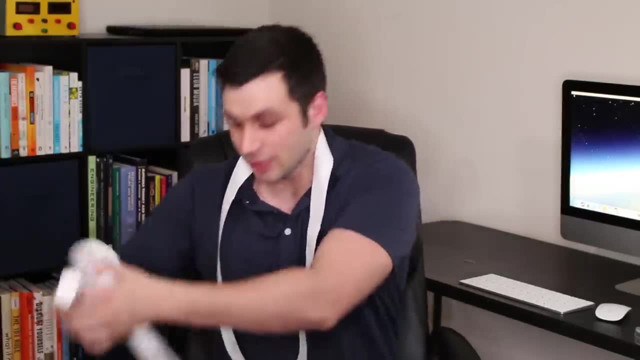 was going to happen the first time i saw this so now you can officially be the life of literally any party you go to and i have nothing left to teach you guys now if you want to know why this happened i'll leave some links below but one thing to think about especially going back to the original mobia strip is how many edges does this have 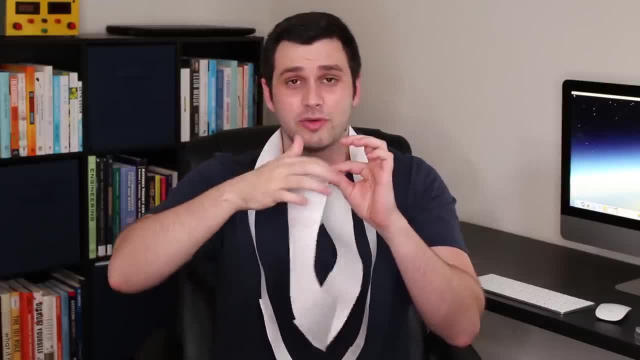 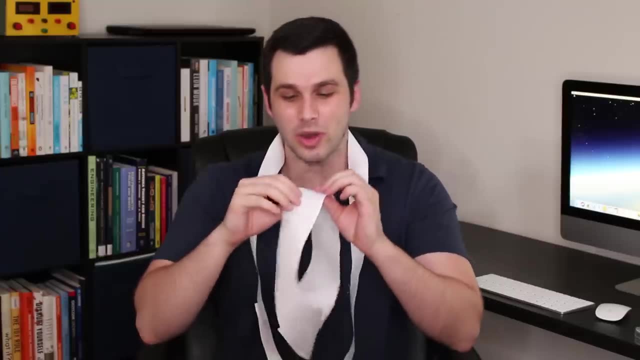 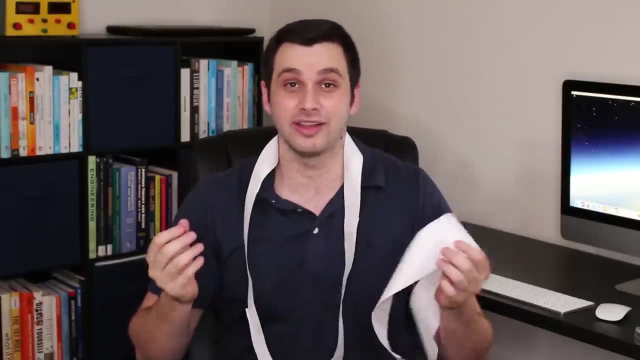 and i'm sure many people will say well there's two you got one over here and one over here but actually it only has one so you got to kind of rethink how you define an edge and then you can start to think about well what happens when i split something in half that only has one edge and it might start to make more sense why you just saw the things that you did 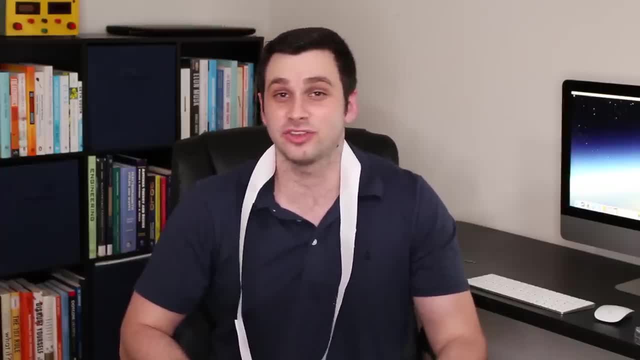 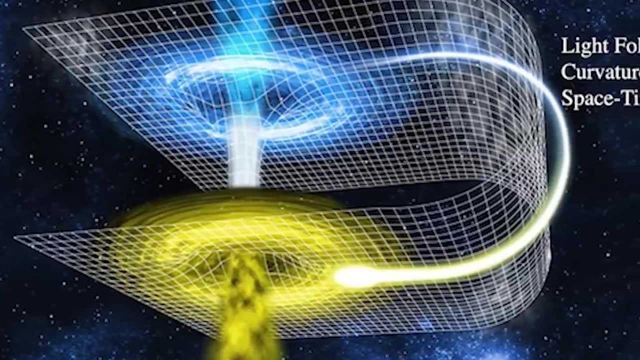 now topology is a pure math class but it does have applications in computer science and computer modeling as well as high levels of physics such as quantum field theory and cosmology as analyzing shapes and properties within those fields and how they work and how they work and how these fields is very math intensive but i just want to acknowledge that in a previous video i 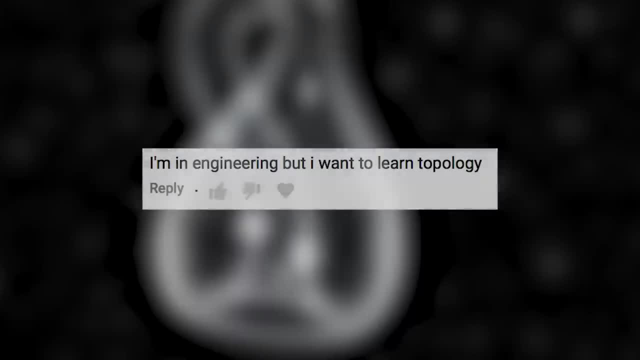 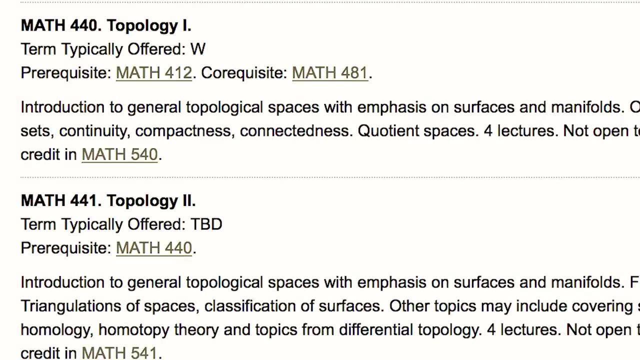 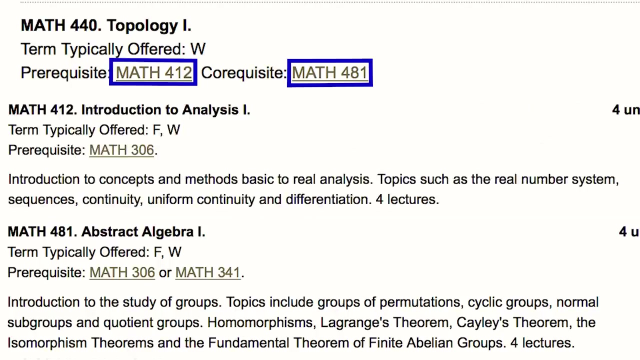 talked about topology and i saw a few comments saying i'm doing engineering but really want to take this class as well i just want to let you know that there are prereqs for this class and at least at my school those included abstract algebra and real analysis which are the pure math classes i said before that really don't have many obvious applications so if you want to get to topology just be prepared for multiple pure math classes first to get there which might mean sacrificing the other math classes if you do get a math minor and also the class will be very math intensive you will not be doing physics and higher dimensions or anything like that it'll be a lot